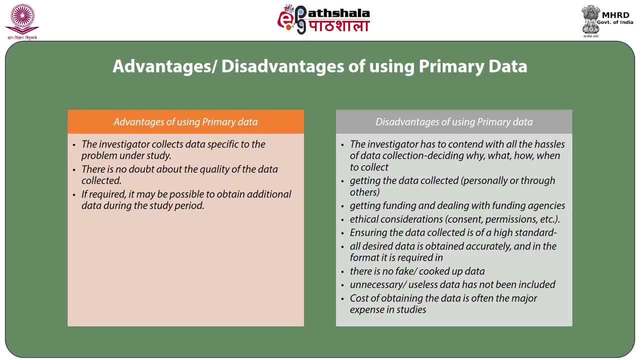 etc. And what are the other disadvantages of using primary data? Ensuring the data collected is of high standard, All desired data is obtained accurately and in the format it is required in. there is no fake or cooked up data. Unnecessary, useless data has not been included. 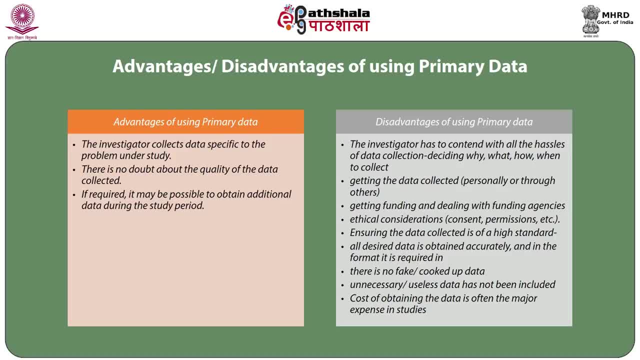 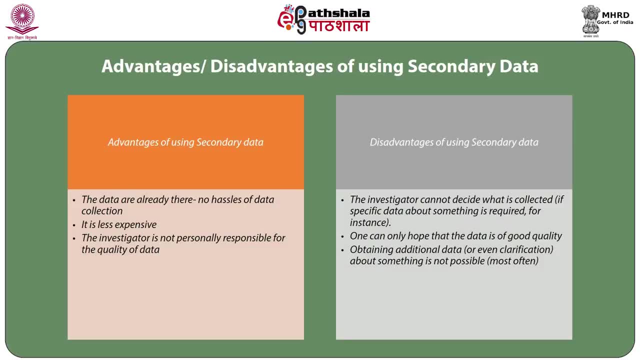 Cost of obtaining the data is often the major expenses in studies. What are the advantages of using secondary data? The data are already there. no hazards of data collection. It is less expensive, Less time consuming. The investigator is not personally responsible for the quality of data. 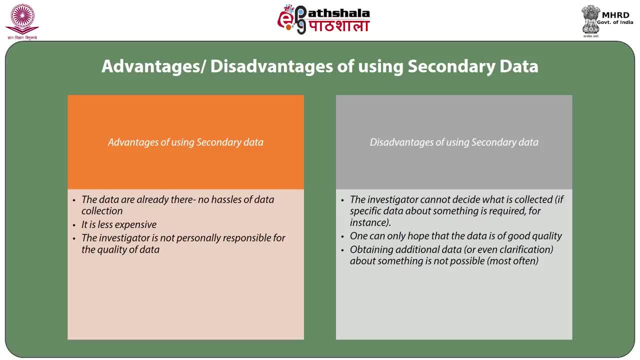 What are the disadvantages of using secondary data? The investigator cannot decide what is collected. The specific data about something is written without any Cruz Quadras and laws. Accommodation is notisin the data that has been collected. The data collected does not differ from the data collected by by market concepts. The data collected is written without. 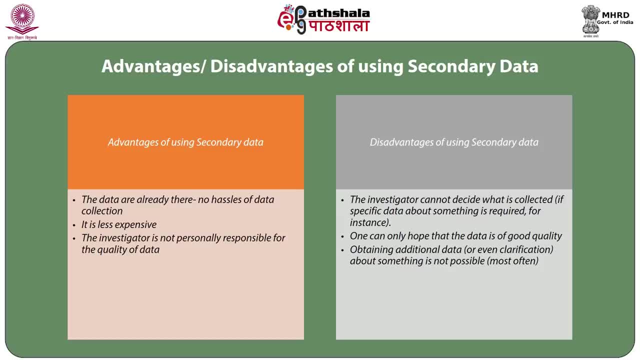 a source. The other way is to collect � common 처� wl which is the data collected white required for instance. One can only hope that the data is of good quality. Obtaining the additional data or even clarification about something is not possible most often. 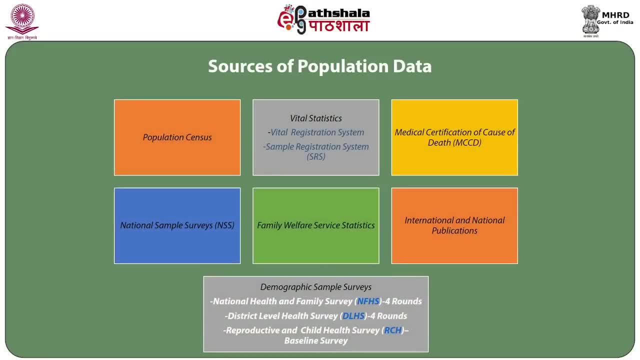 Then, coming to the sources of population data, The data are obtained mainly through population census. Then, second one is vital statistics. Under vital statistics, we have Vital Registration System and Sample Registration System. The third one is Medical Certification of Cause of Death. Then fourth one is National Sample Surveys. Fifth one is Demographic. 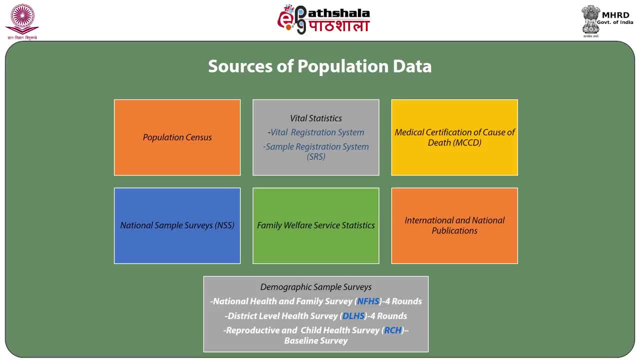 Sample Surveys. Under Demographic Sample Surveys we have National Health and Family Survey, District-Level Health Survey, Pre-Productive and Child Health Surveys, Baseline Surveys, Then Family Welfare Service Statistics, then, last but not least, International and National. 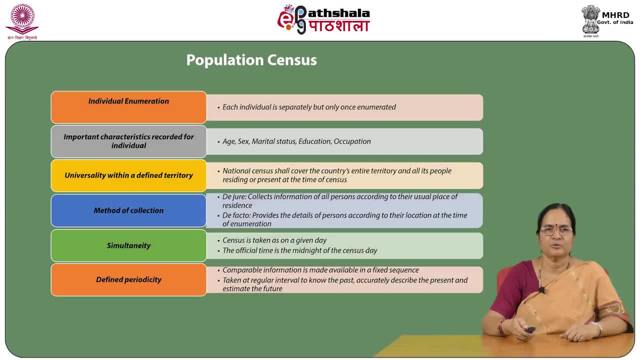 Publications. Coming to population census, it is the most important source of data. The purpose is to produce data on various aspects of population: demographic, economic, social data pertaining to all persons in a country or in a well defined part of a country at a specified time. So 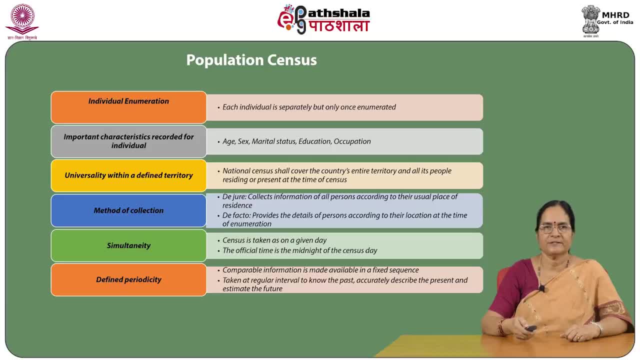 population census has some specific use cases. Special Features: No 1 is Individual Enumeration. Each individual is separately, but only once, enumerated. Some important characteristics of each person are separately recorded, like age, sex, marital status, education, occupation, etc. The third important feature is Universality within a defined territory. 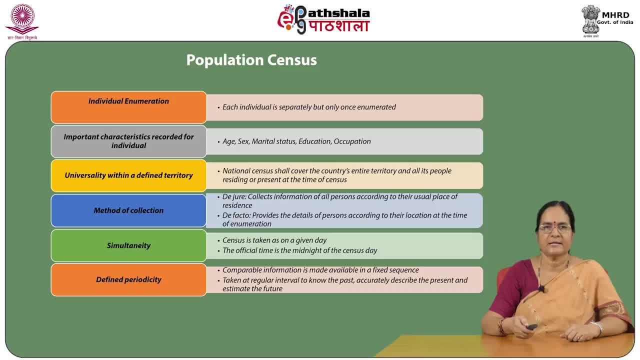 National census shall cover the country's entire territory and all its people residing or present at the time of survey. What are the methods of collection? There are two important methods of collection: D0 and D-FACTO. D-0 means collects information of all persons according to their usual place of residence. 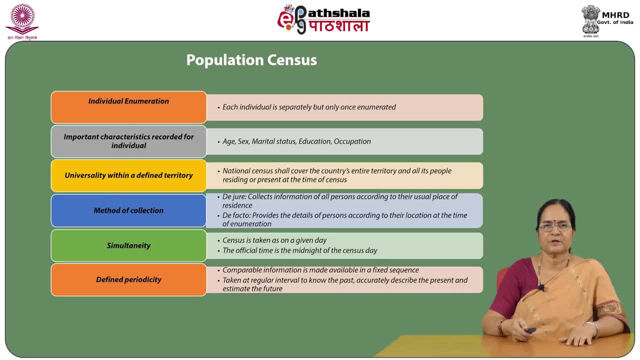 D-FACTO method provides the details of persons according to their location. D-FACTO method provides the details of persons according to their location. D-FACTO method provides the details of persons according to their location Simultaneously is another special feature of the census. 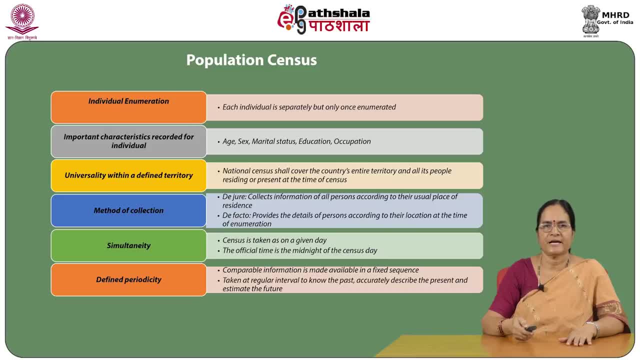 Census is taken as on a given day, The official time is the midnight of the census day, Then defined periods. day Census should be taken at regular intervals, ie every 10 years. Comparable information is made available in a fixed sequence. A series of census makes it possible to know the past accurately, describe the present. 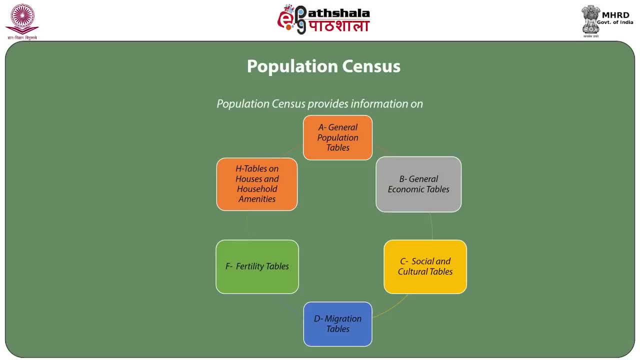 A series of census makes it possible to know the past accurately. describe the present. A series of census makes it possible to know the past accurately. describe the present. estimate the future. census provides information in a series: a series gives general population tables. b series gives general economic tables. c tells about social and cultural tables, d about 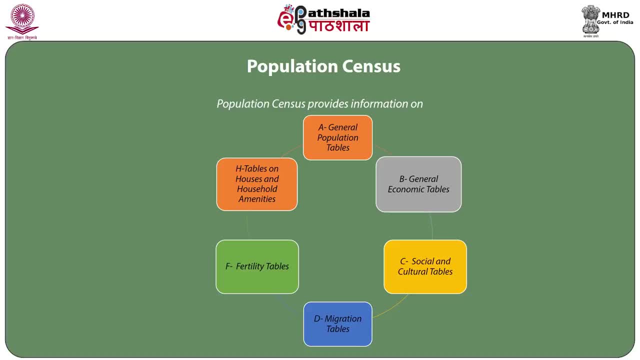 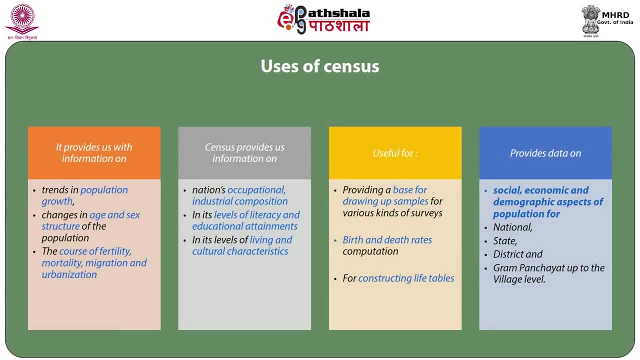 migration. tables f is confined to fertility. tables h tables on houses and household amenities. what are the uses of census? it provides us with an information on trends in population growth, changes in age and sex structure of the population, the course of fertility, mortality, migration and urbanization. census provides us information on nation's occupational industrial composition. 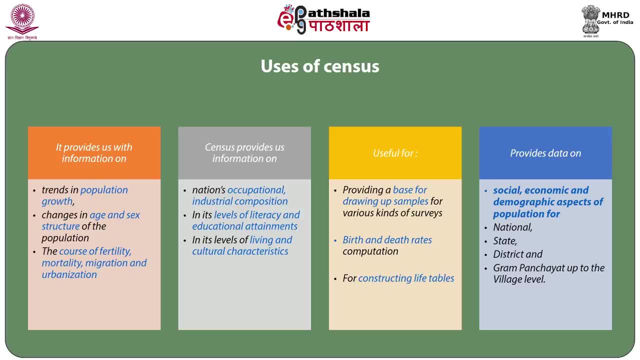 in its level of literacy and educational attainments, in its level of living and cultural characteristics. what are the other uses of census? it's useful in providing a base for drawing up samples for various kinds of surveys. births and death rates can be computed. census data are useful for constructing life tables. census day. 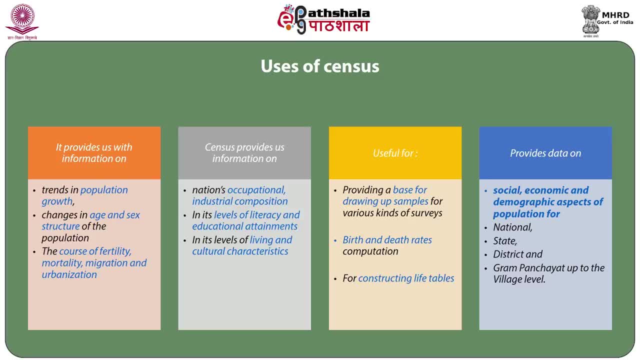 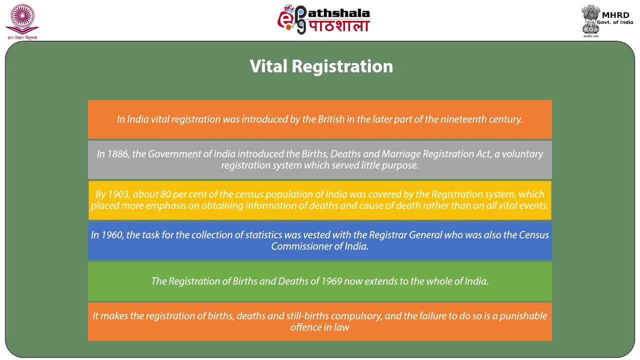 provides data on social, economic, demographic aspects of population per national state district in gram panchayat up to village level. then comes to the second important source of data: vital visitation in india. the system of vital registration was introduced by the british in the later part of. 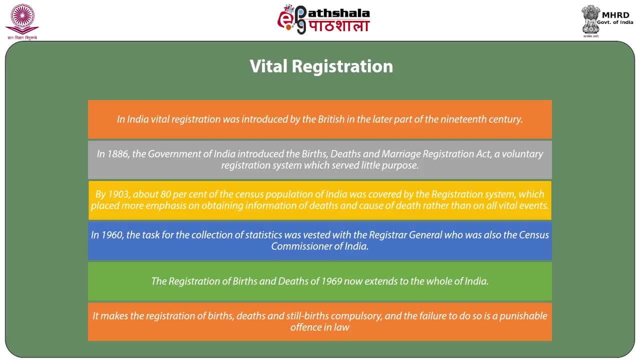 century. in eighteen eighty six, the government of independently sent on up to death orgal le piaget risonar. in nineteen sixty, detype for collection of statistics was vested with the registrar general, who was also the census commissioner of India. The registration of births- deaths of 1969 now extends to the whole of India. 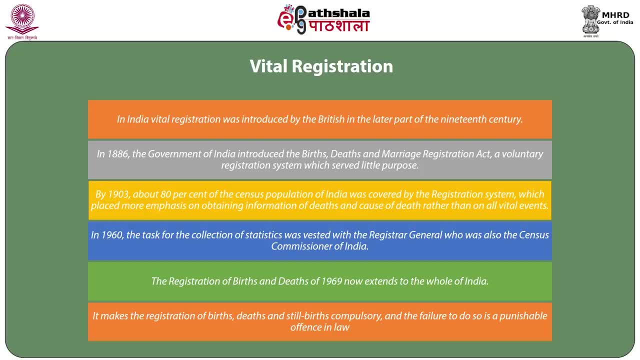 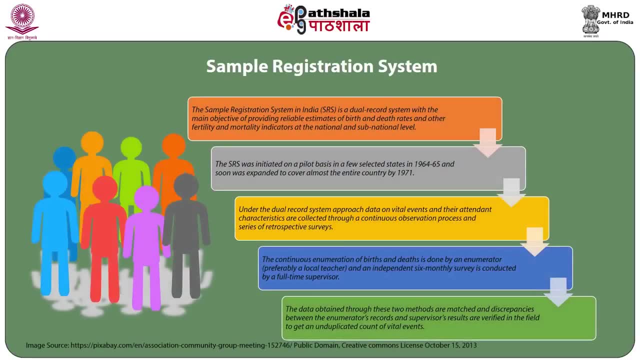 It makes the registration of births, deaths and still births compulsory, and the failure to do so is punishable offense in law. Then comes to sample registration system. SRS, The sample registration system in India is a dual record system with the main objective of providing reliable estimates of birth. 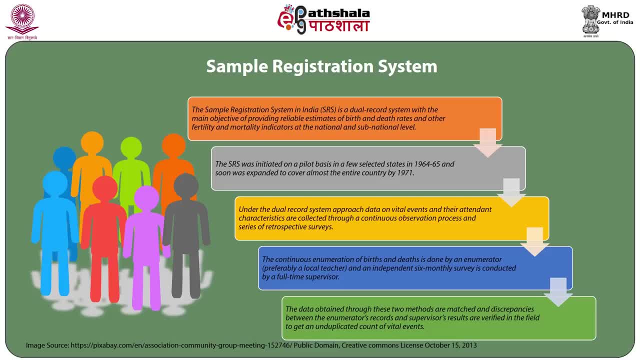 and death rates and other fertility and mortality indicators at the national and sub national level. The SRS was initiated on a pilot basis in a few selected states in 1964-65 and soon was expanded to cover almost the entire country by 71.. Under dual record system approach, data on vital events. 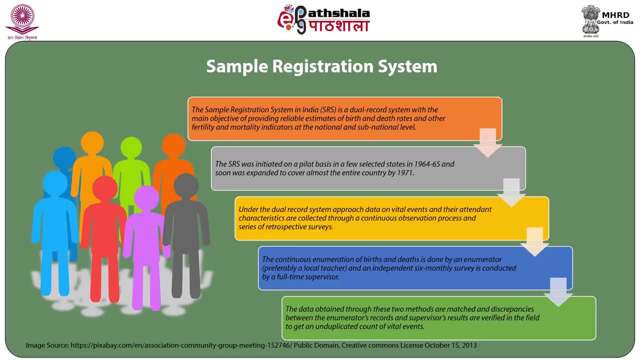 and their outcomes. further studies have been conducted to understand the importance of racial differences and sub national levels. The SRS also considers the impact of帶s and carbon, and other Attendant characteristics are collected through a continuous observation process and series of retrospective surveys. 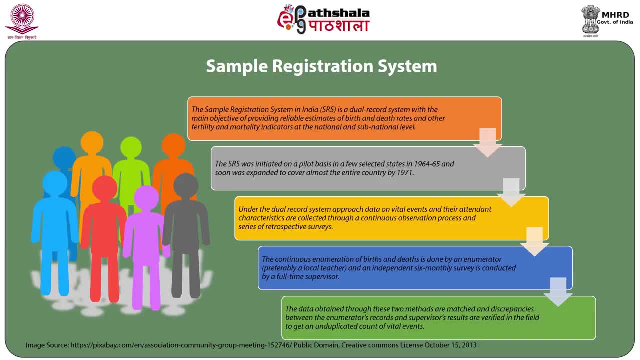 The continuous enumeration of births and deaths is done by an enumerator, preferably a local teacher, and an independent six-monthly survey is conducted by a full-time supervisor. The data obtained through these two methods are matched and discrepancies between the enumerator's reports and the supervisor's results are verified in the field to get an unduplicated count of vital events. 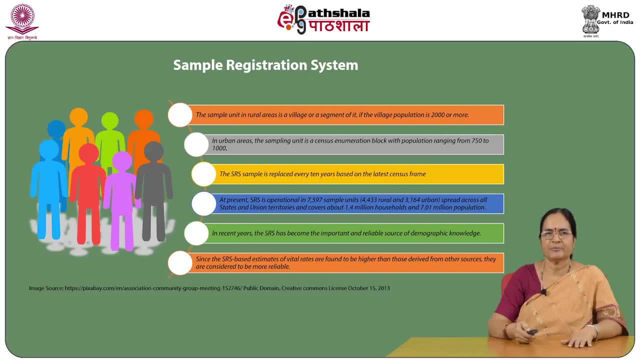 The sample unit in rural areas is a village or a segment of it, if the village population is 2,000 or more. In urban areas, the sampling unit is a census enumeration block with population ranging from some 50 to 1,000.. 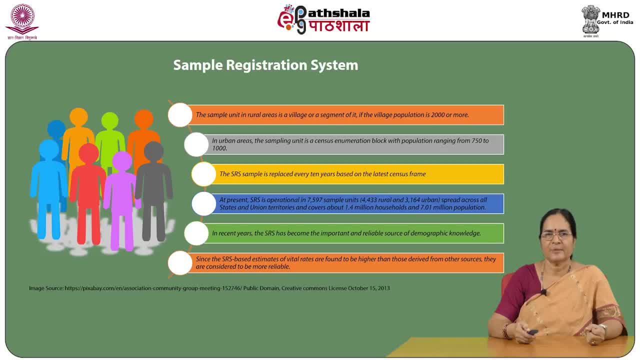 The SRS sample is replaced every 10 years based on the latest census frame. At present, SRS is operational in 7,597 sample units, 4,433 rural and 3,164 urban, spread across all states and union territories and covers about 1.4 million households and 7.01 million population. 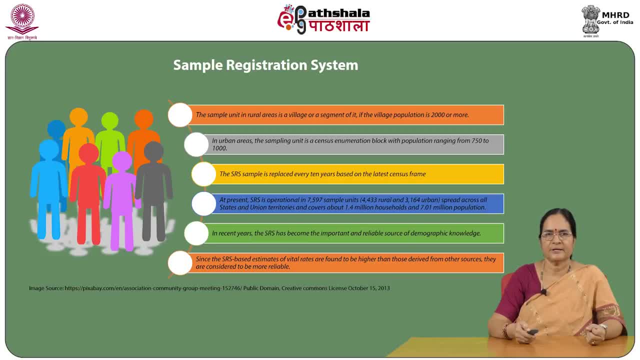 In recent years the SRS became the important source of demographic knowledge. Since the SRS-based estimates of vital rates are found to be higher than those derived from other sources, they are considered to be more reliable. But the limitation is it gives only the data back, 2 years back data. 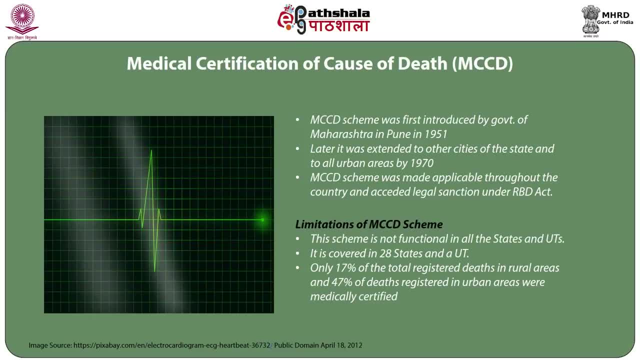 Medical Certification of Cause of Death- MCCD. MCCD scheme was first introduced by Government of Maharashtra in Pune In 1951, later it was extended to other cities of the state and to all urban areas by 1970.. MCCD scheme was made applicable through the country and exceeded legal sanction under RBD Act. 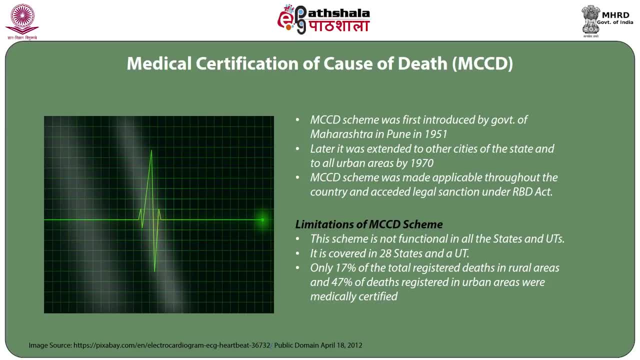 But it has some limitations. This scheme is not functional in all the states and union territories. It covered, in 28 states and a union territory, Only 17% of the total registered deaths in rural areas And 47% of the total registered deaths in rural areas. 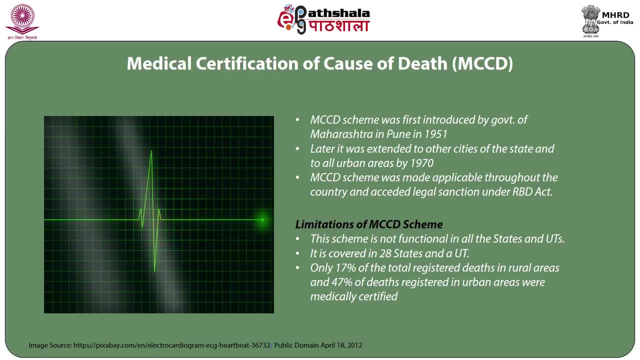 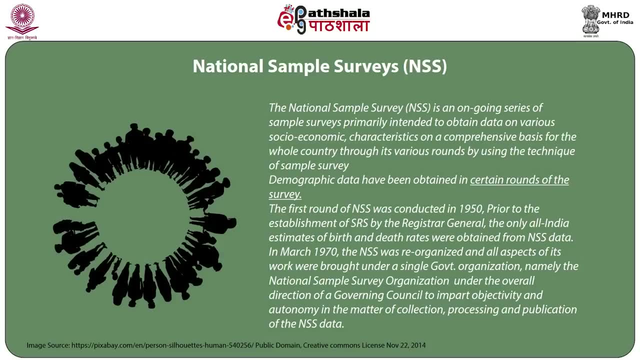 And 47% of the total registered deaths in urban areas were medically certified. National Sample Survey. The National Sample Survey is an ongoing series of sample surveys primarily intended to obtain data on various socio-economic characteristics on a comprehensive basis for the whole country through its various rounds, by using the technique of sample survey. 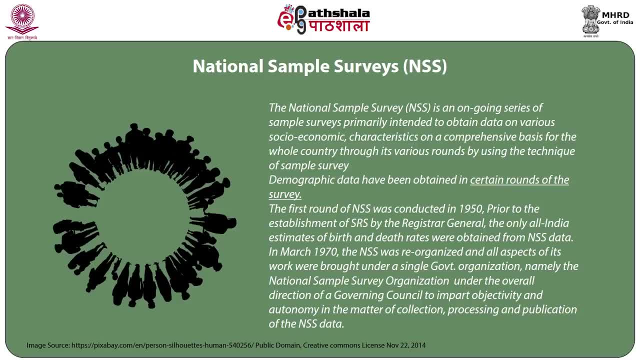 Demographic data have been obtained in certain rounds of the survey. The first round of NSS was conducted in 1950.. Prior to the establishment of SRS by the Registered General, the only all-Indian estimates of birth and death rates were obtained from NSS data. 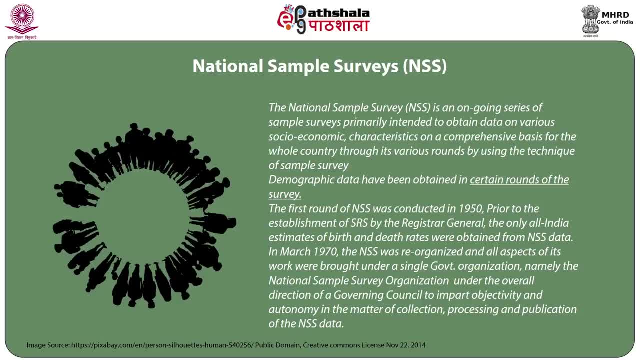 the only all-Indian estimates of birth and death rates were obtained from NSS data. In March 1970, the NSS was reorganized and all aspects of its work were brought under a single Government organization, namely the Natural Sample Survey organization, Under the overall direction of a governing council. 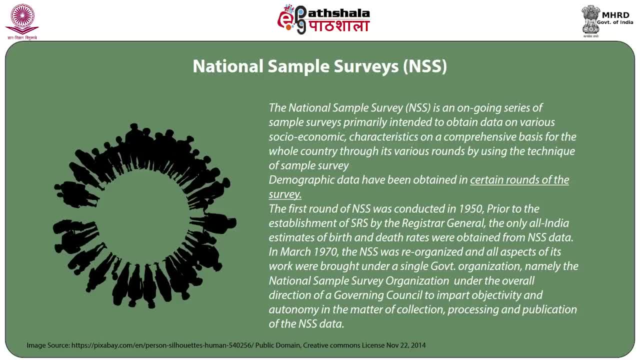 to import the objective sample and blood test samples for data. To import the objective sample group and cancer pridepar. the NSS data was searched by��았as and universally and ethically versucht to get data productivity and autonomy in the matter of collection, processing and publication of. 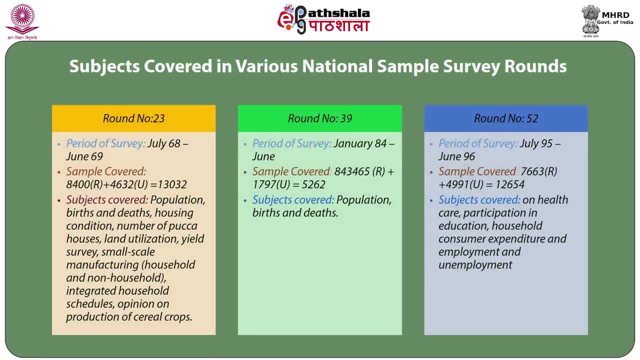 the NSS data Subjects covered in various national sample survey rounds In round number 23,. period of survey is July 68 to June 69,. sample covered was 8,400 rural and 4,632 urban. Subjects covered are population, births and deaths, housing condition, number of pakka. 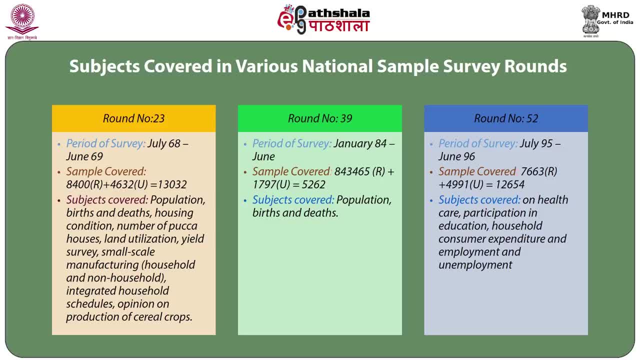 houses: land utilization yield survey. small-scale manufacturing. household and non-household integrated household schedules. opinion on production of cereal crops. The other rounds like round number 39,. period of survey: January 84 to June. sample covered 4,043,065 rural and 1,797 urban. 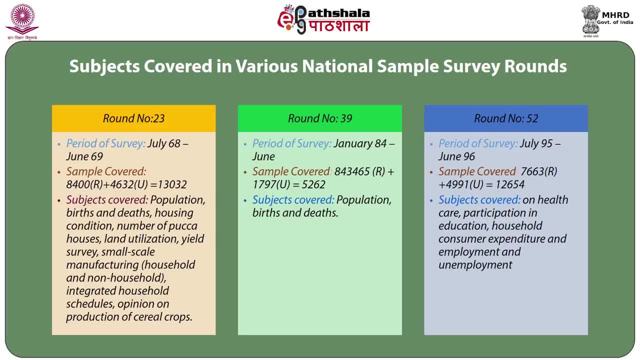 In round number 52, period of survey: July 95 to June 96,. sample covered: 12,654, with 7,663 rural and 4,991 urban. Subjects covered on healthcare, participation in education, household consumer expenditure and employment and unemployment. Subjects covered in round number 52, period of survey: July 95 to June 96,. sample covered: 12,654, with 7,663 rural and 4,991 urban. Then comes the Demographic Sample Surveys, a large-scale and benchmark demographic sample. 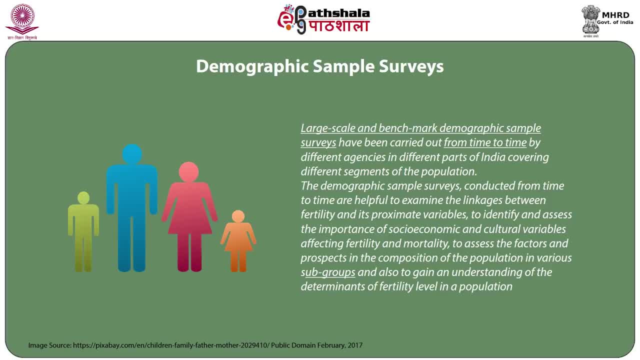 surveys have been carried out from time to time by different agencies in different parts of India, covering different segments of the population. The demographic sample surveys conducted from time to time are helpful to examine the linkages between fertility and its proximate variables, to identify and assess the importance of socio-economic 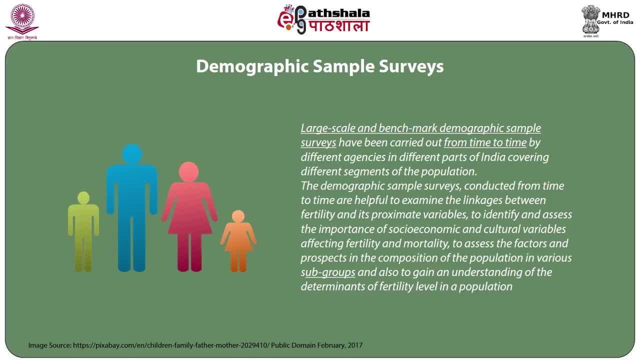 and cultural variables. Subjects covered on healthcare, participation in education, household and non-household cultural sustainability and business maintenance in human rights. The demographic sample was Ägbeman Space 15. ij 19.. In ë, Jerusalem aged 21: 10 ë barrier age of shuttle. seventy four ë wine age of. 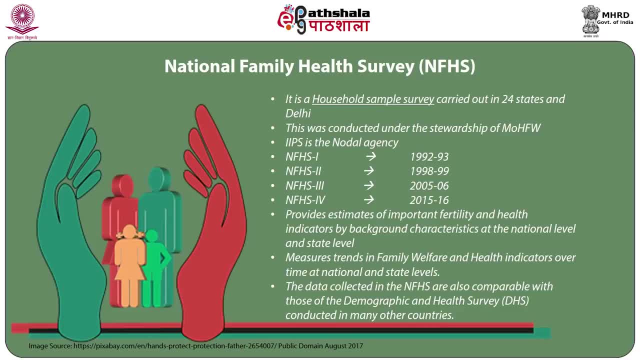 twenty two ë Neils Fil mier, age of ten to twenty-two. indicators: ë주고ge ë recognition, ë achievement ë, ë health, ë innovation, ë memory ë and ë healthë in province. 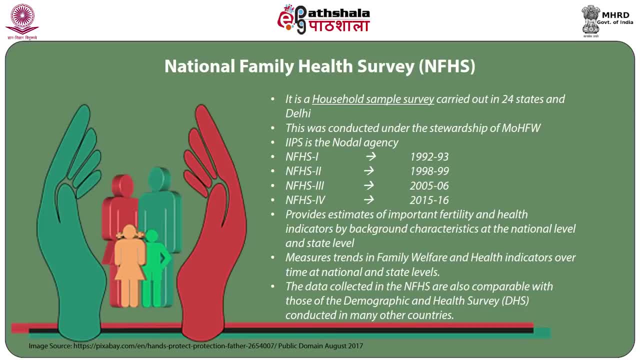 The density populationemand ëmanyí assessment of age subway population. The populationás conversation was being very active and active during ëYenikí in ëishing ë D s港 Service. úK 해awaííí ï Bird på ê ð æ Krudaíííííííííííííííííííííííííííííííííííííþä configuration. 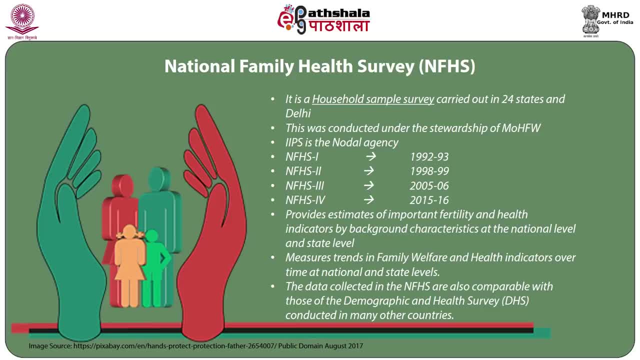 is the nodal agency. NFHS-1 was conducted in 92-93,, NFHS-2 in 98-99,, NFHS-3 in 2005-06 and NFHS-4 in 2015-16.. First, NFHS-1 and NFHS-2 were conducted in every 5 years, whereas NFHS-3. 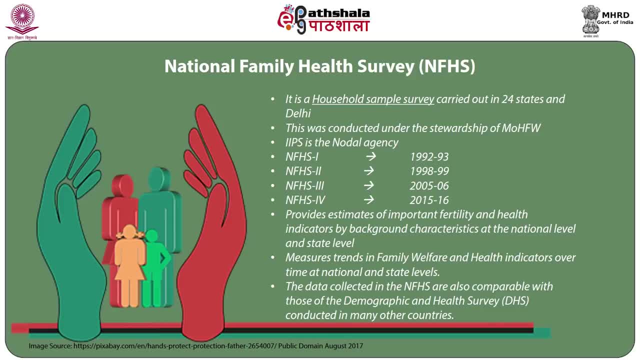 and 4 were conducted once in 10 years. This NFHS provides estimates of important fertility and health indicators by background characteristics at the national level and state level. measure trends in family welfare and health indicators over time at national and state levels. The data: 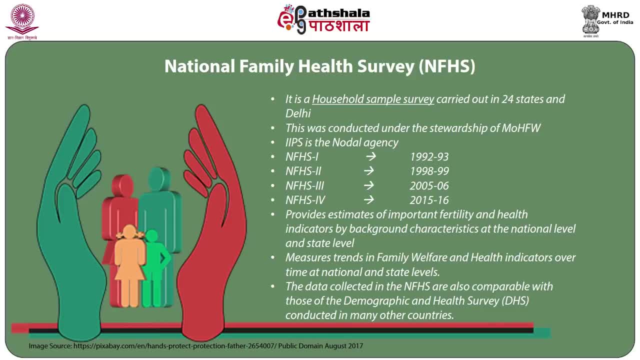 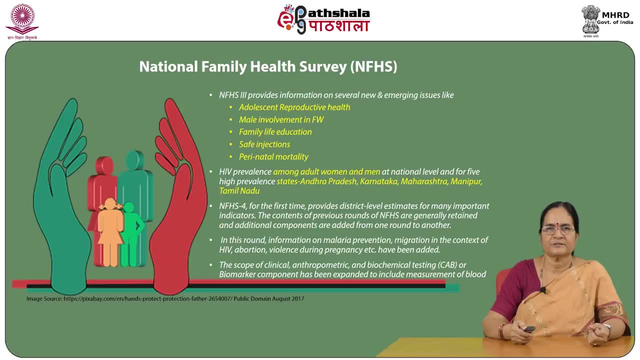 collected in NFHS are also comparable with those of the demographic and health surveys conducted in many other. NFHS-3 provides information on several new and emerging issues like adolescent reproductive health, main involvement in family welfare, family life, education, safe injections, perinatal. 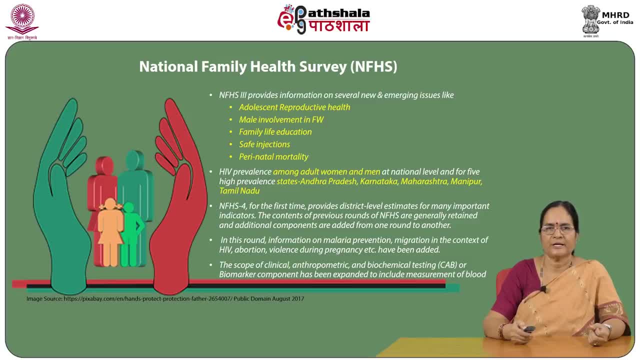 mortality, HIV prevalence among adult women and men at national level and for 5 high prevalence states like Andhra Pradesh, Karnataka, Maharashtra, Manipur and Tamil Nadu. NFHS-4, for this first time, provides statistics on the number of cases of HIV in the country. The data collected: 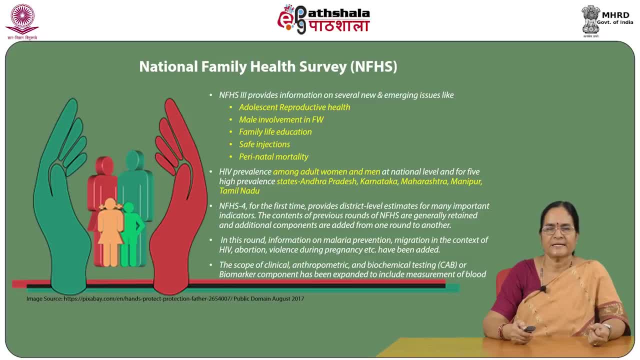 in this second round provides a good statistic level estimates for many important indicators. The contents of previous rounds of NFHS-3 are generally retained and the additional components are added from one round to another. In this round: information on malaria prevention, migration in the context of HIV, abortion. 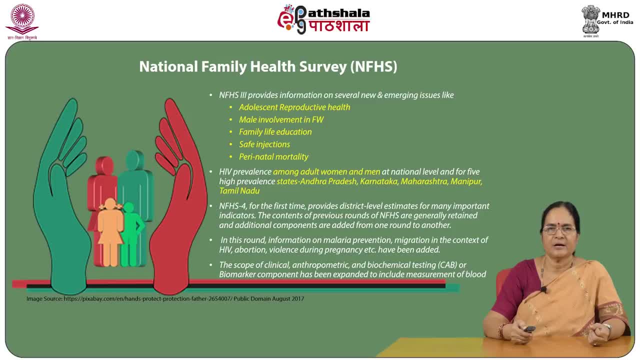 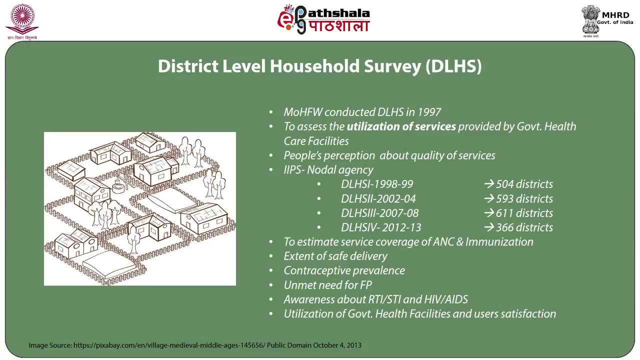 violence during pregnancy, etc. have been added. The scope of clinical anthropometric and biochemical testing- CAB or Bio maker component- has been expanded to include measurement of blood pressure and blood glucose levels. The other survey is district level household survey, DLHS. Ministry of Health and Family Welfare conducted DLHS in 1997 to assess the utilization of 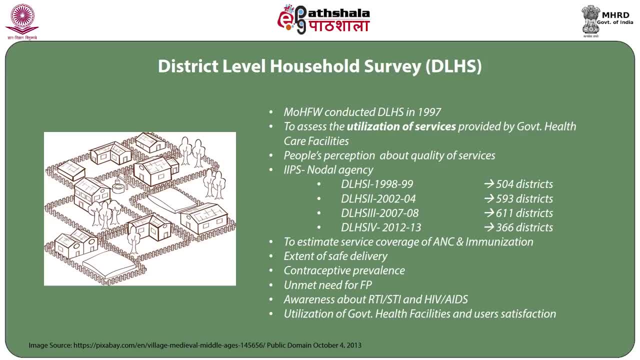 services provided by government of healthcare facilities for people's perceptions about quality of services, and International Institute for Population Sciences is the nodal agency. DLHS 1 was conducted in 1998-99 in 504 districts. DLHS 2 was conducted in 2002-04 in 593 districts. 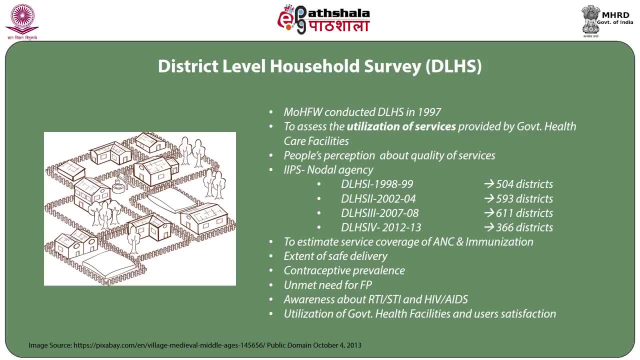 DLHS 3 was conducted in 2007-08 in 611 districts, whereas DLHS 4 was conducted in 2012-13 in 366 districts. From DLHS 1 to 2, 2 to 3,, they have expanded the districts. 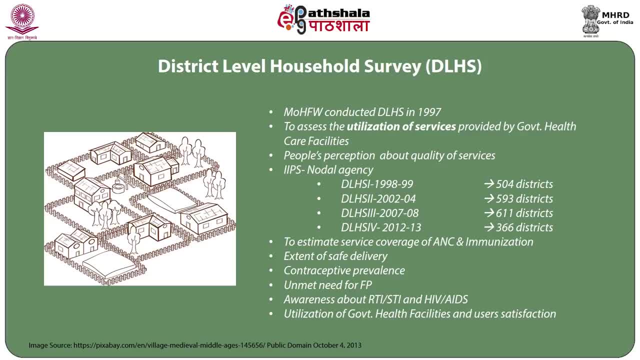 Whereas in DLHS 4, they have concentrated on the quality of the information collected and they have collected in a limited number of districts, that is, 366 districts In district level household survey. the main objectives are to estimate service coverage of ANC and immunization. extent of safe delivery, contraceptive prevalence, unmet need for family. 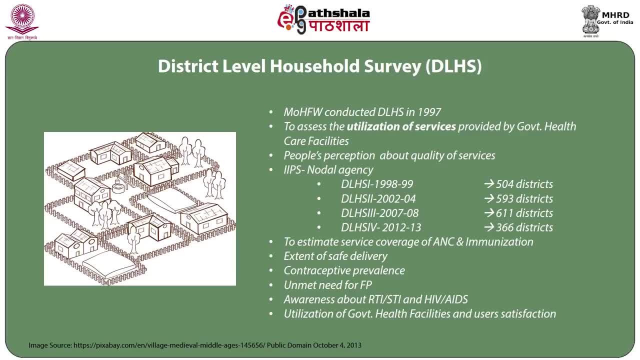 planning, awareness about RTI, STI and HIV-AIDS. The main objectives are to estimate the service coverage of ANC and immunization. extent of safe delivery, contraceptive prevalence. unmet need for family planning, awareness about RTI, STI and HIV-AIDS. 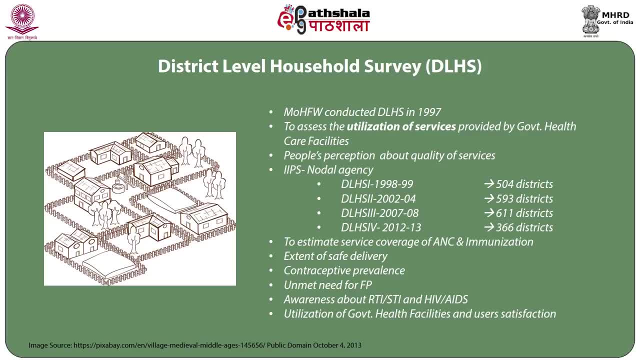 The main objectives are to estimate the service coverage of ANC and immunization, extent of safe delivery, contraceptive prevalence, unmet need for family planning, awareness about RTI, STI and HIV-AIDS, Utilisation of government health facilities and users satisfaction. 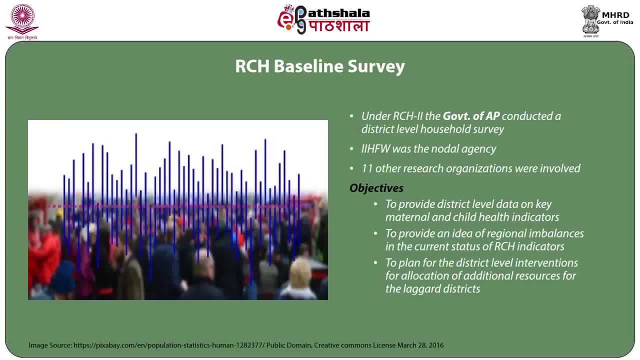 In RCH Baseline survey. under RCH 2,, the Government of Andhra Pradesh conducted a district level household survey. Indian Institute of Health and Family Welfare was the nodal agency. eleven other research organizations were involved. The objectives are to provide district level data on key maternal and child health indicators. 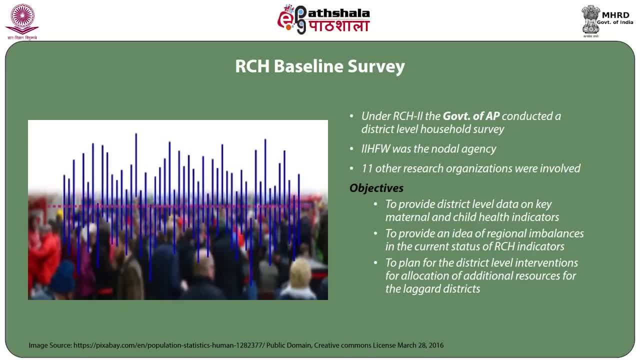 to provide an idea of regional impact and the review for social engagement in the home health system. The objectives are to provide district level data on key maternal and child health indicators, balances in the current status of RCH indicators and to plan for district level interventions. 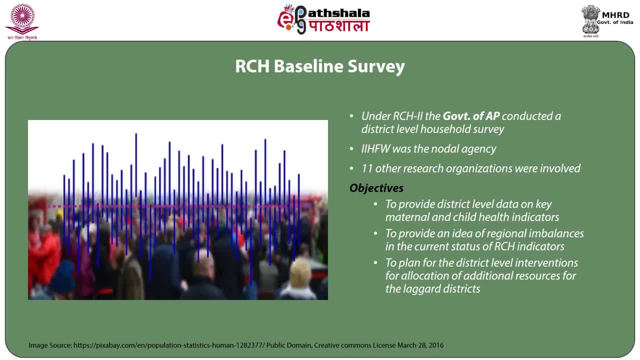 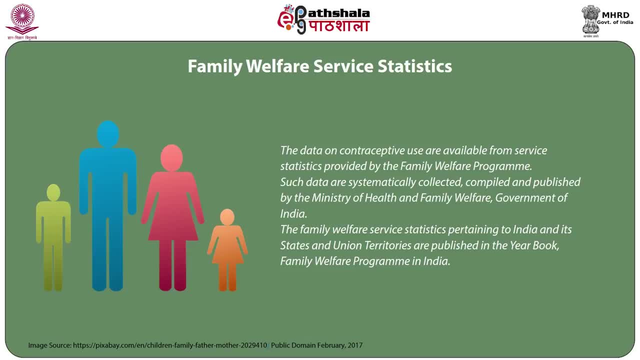 for allocation of additional resources for the laggard districts. Then comes the another source of population data: Family Welfare Service Statistics. The data on contraceptive use are available from service statistics provided by the Family Welfare Program. Such data are systematically collected, compiled and published by the Ministry of Health and 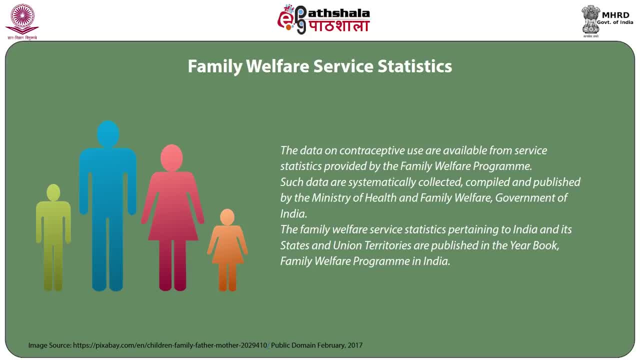 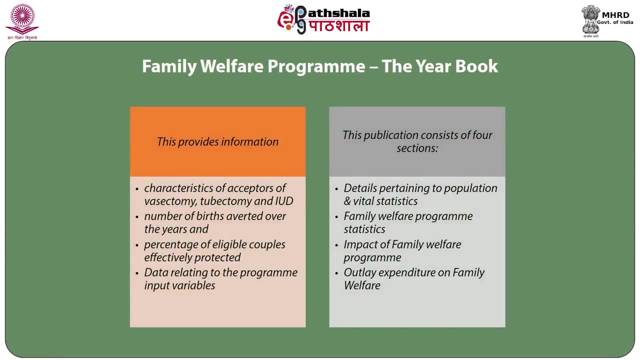 Family Welfare Government of India. The Family Welfare Service. Statistics pertaining to India and its states and union territories are published in the yearbook called Family Welfare Program in India. This Family Welfare Program in India- the yearbook. this provides information on characteristics of acceptors of vasectomy, tuvectomy and IUD, number of births awarded over the years and 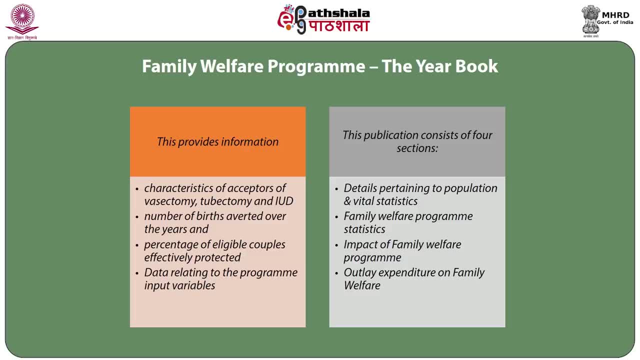 the percentage of eligible couples Effectively protected. data relating to the program input variables. This Family Welfare Program: the yearbook. this publication consists of four sections: details pertaining to population and vital statistics. Family Welfare Program statistics. impact of Family Welfare Program Outlay expenditure and Family Welfare. 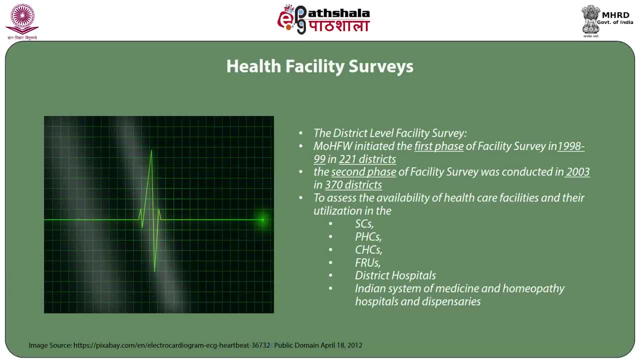 Health Facility Survey- The district level facility survey. The district level facility survey Was conducted by Ministry of Health and Family Welfare and initiated the first phase of facility survey in 1998 and 1999 in 221 districts. The second phase of facility survey was conducted in 2003 in 370 districts. 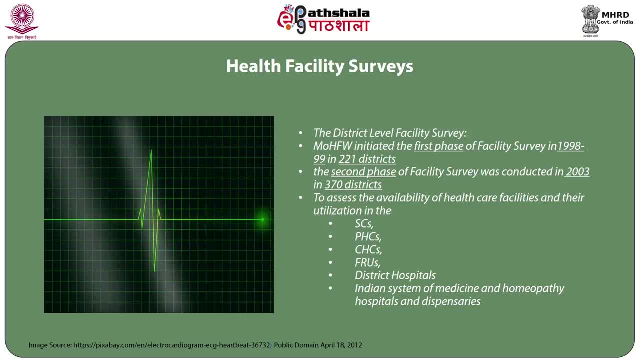 What are the objectives of this Health Facility Survey? To assess the availability of health care facilities and their utilization in the sub-centres: primary health centres, community health centres, first referral units, district hospitals, health facilities, Community health centres, Indian system of medicine and homeopathy hospitals and dispensaries. 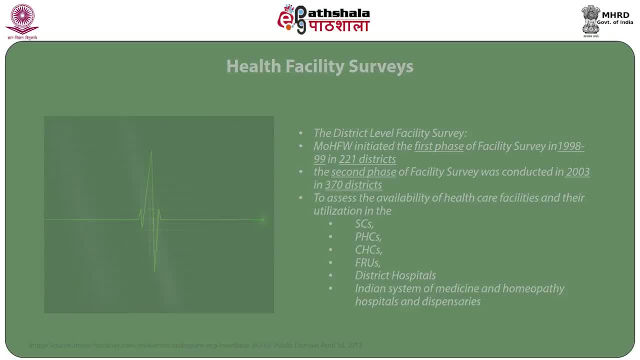 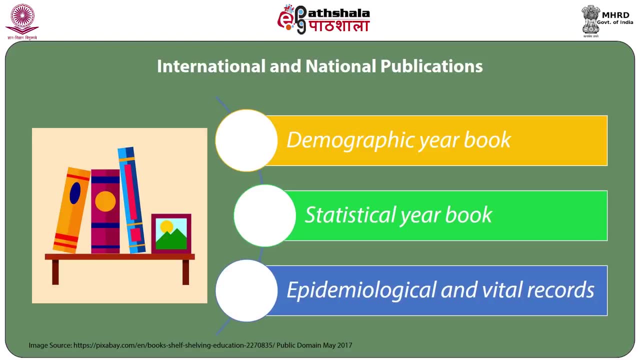 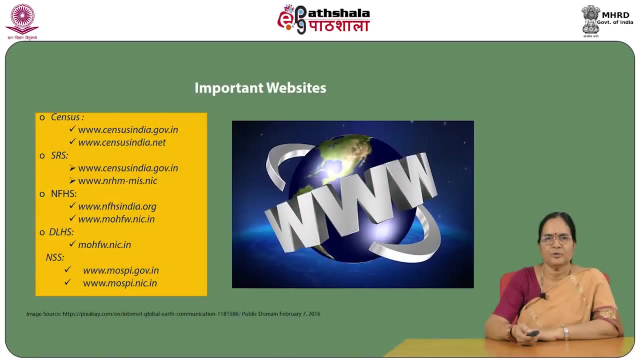 Community health centres, Indian system of medicine and homeopathy, hospitals and dispensaries. The last source of data is International and National Publications. There are Demographic Yearbooks, Statistical Yearbooks and Epidemiological Vital Records. There are some important websites. if you want to see the census information, you can. 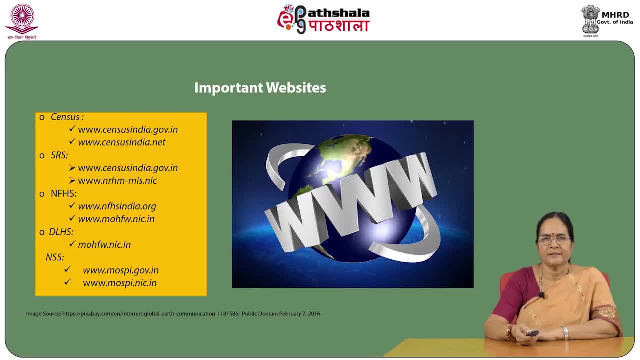 go to wwwcensusindiagovin, Thank You. Thank you of govin wwwcensusindianet. If you want to go for the SRS sample registration system, you can visit the website wwwcensusindiagovin- wwwnrhm-misnic For NFHS information. 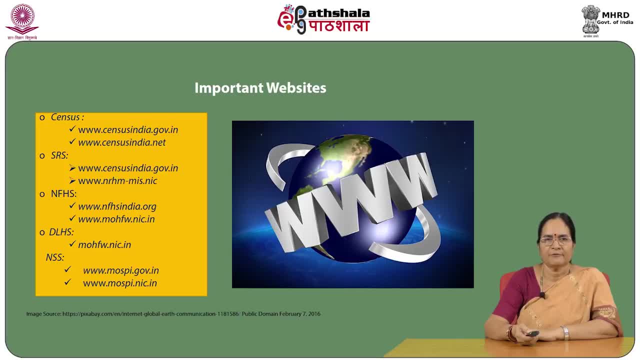 you can go to wwwnfhsindiaorg. wwwmohfwnicin For DLHS information. you can visit the website wwwmohfwnicin For NSS: wwwmospigovin, wwwmospinicin. 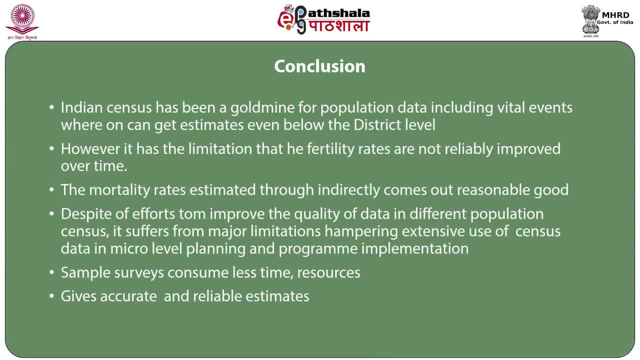 For concluding the population data sources. we can say we can highlight the important findings. like Indian, census has been a gold mine for population data, including vital events, where one can get estimates even below the district level, up to village level we can get the information. However, it has the limitation that fertility rates are not reliably improved. 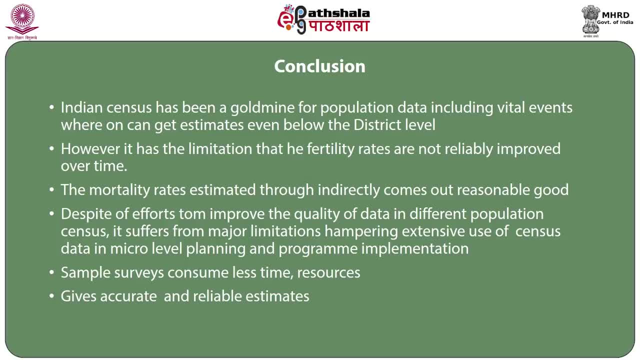 over time. Quality rates estimated through indirectly comes out reasonably good using the census data. Despite of efforts to improve the quality of data in different population census, it suffers from major limitations hampering extensive use of census data in micro level planning and program implementation. 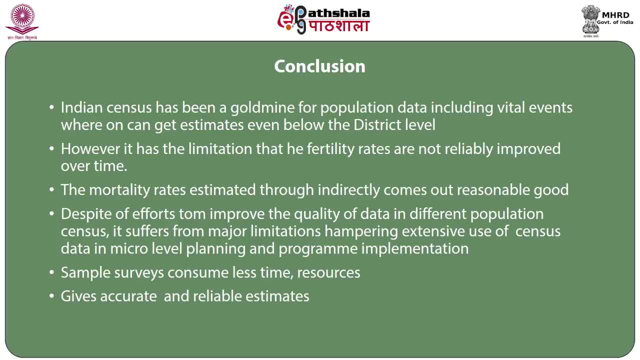 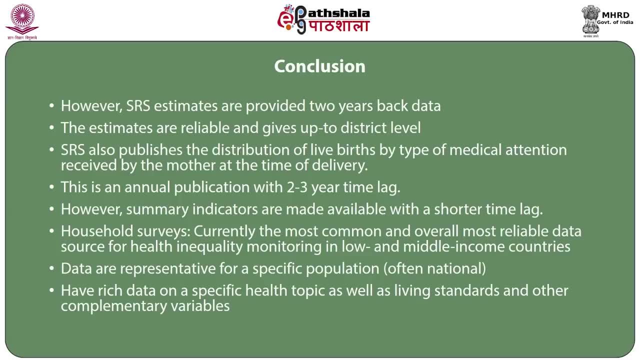 Coming to sample surveys. sample surveys consume less time resources. gives accurate and reliable estimates. However, SRS estimates are provided 2 years back data. The estimates are reliable and gives up to district level. SRS also publishes the distribution of libors by type of medical attention received by mother.